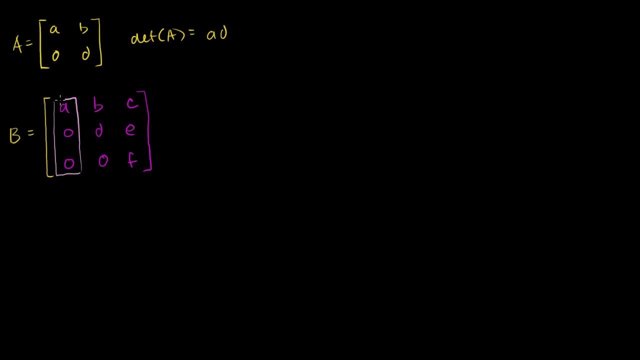 So let's find the determinant along this column right here. So the determinant of b is going to be equal to a times the submatrix, if you were to ignore a's row and column. So a times the determinant of d, e, 0, f. 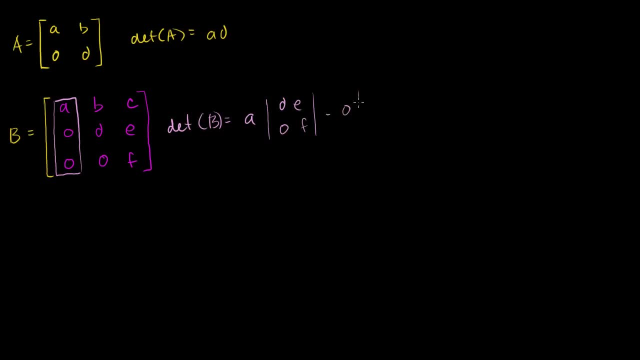 And then minus 0 times its determinant of its submatrix. that row and that column, you get b, c, 0, f, And then you have plus 0 times, you get rid of that row and that column. you get b, c, d, e. 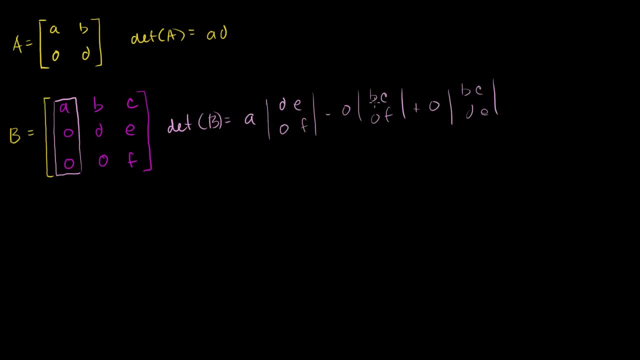 Now, obviously, these two guys are going to be 0.. I don't care what these 2 by 2 matrices, what their determinants end up evaluating to, So these are both going to be equal to 0, because we're multiplying by 0.. 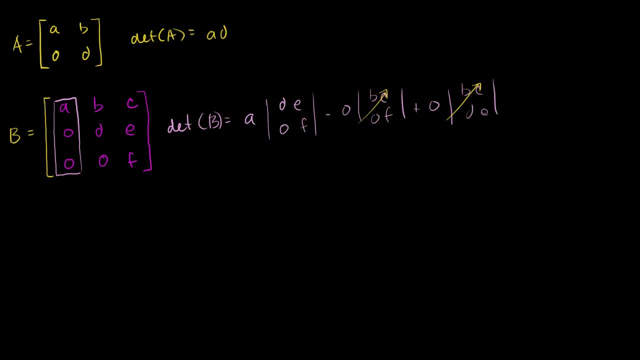 We're left with a times the determinant of this. And the determinant of this is pretty straightforward. We're going to have. it's going to be equal to a times. the determinant of this is d f, d f minus 0 times e. 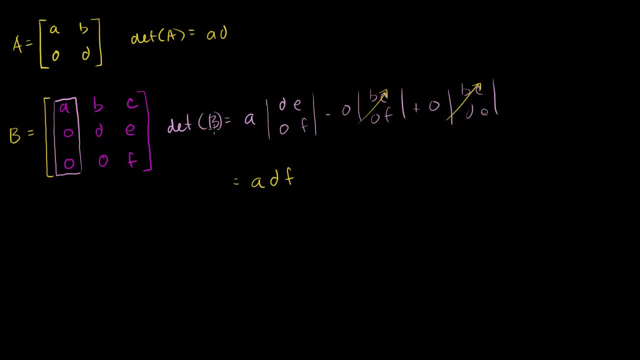 So it's just going to be d- f. So the determinant of b is a, d, f. Notice the determinant of a was just a and d. Now you might see a pattern. In both cases we had 0's below the main diagonal. 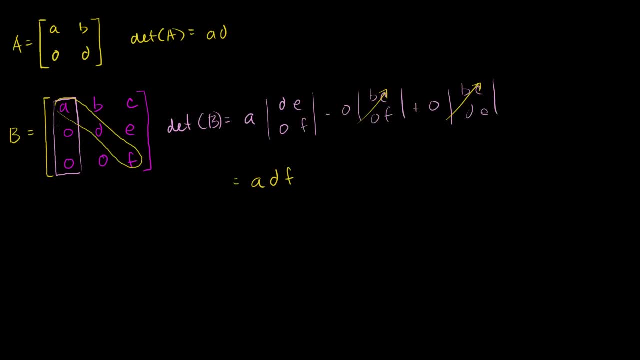 This was the main diagonal right here, And when we took the determinants of the matrix, the determinant just ended up being the product of the entries along the main diagonal, And if you think that that's a general trend that always applies, you are correct. 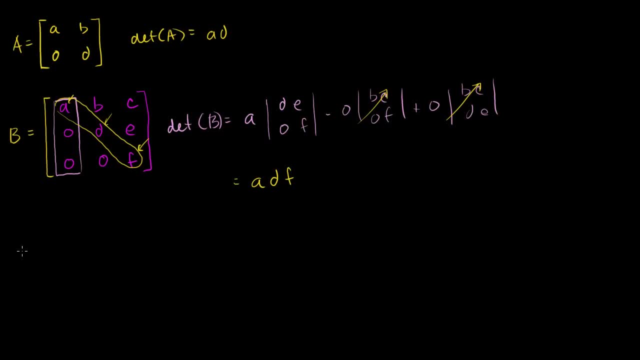 We can do it in the general case. Let's do the general case. So let's say we have some matrix A and it is equal to a 1, 1.. Then you have a 2, 2.. You're going to have a 0, right there. 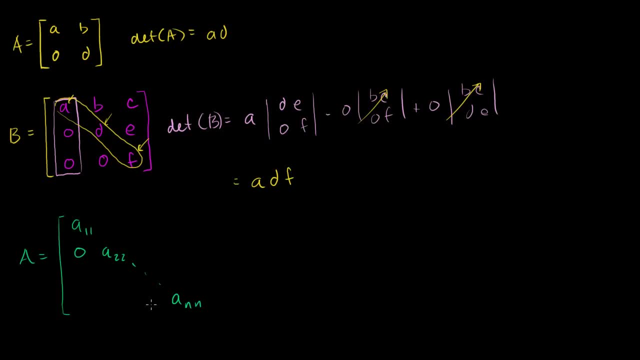 And then you just keep going all the way down to a n, n In this row, everything is going to be a 0. 0. 0. 0.. Everything's going to be a 0, except for that last column. 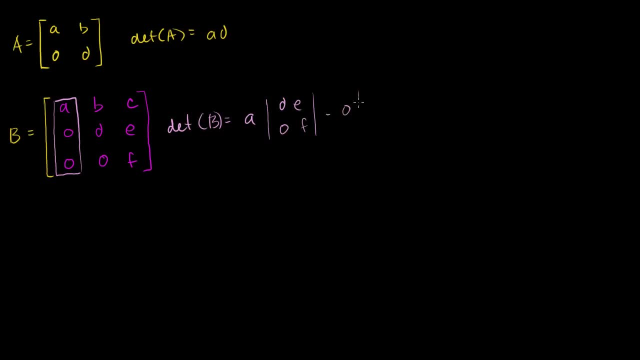 And then minus 0 times its determinant of its submatrix. that row and that column, you get b, c, 0, f, And then you have plus 0 times, you get rid of that row and that column. you get b, c, d, e. 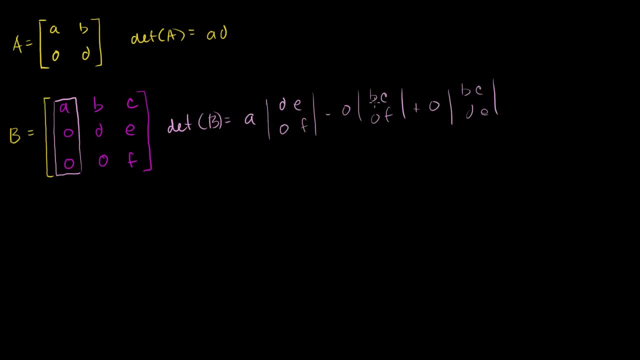 Now, obviously, these two guys are going to be 0.. I don't care what these 2 by 2 matrices, what their determinants end up evaluating to, So these are both going to be equal to 0, because we're multiplying by 0.. 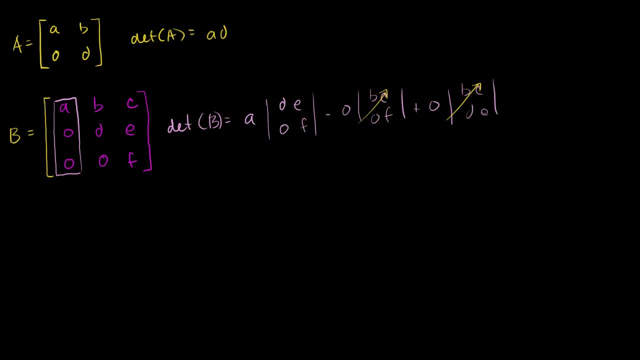 We're left with a times the determinant of this. And the determinant of this is pretty straightforward. We're going to have. it's going to be equal to a times. the determinant of this is d f, d f minus 0 times e. 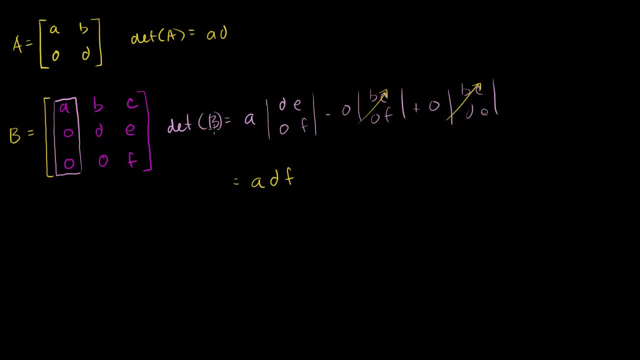 So it's just going to be d- f. So the determinant of b is a, d, f. Notice the determinant of a was just a and d. Now you might see a pattern. In both cases we had 0's below the main diagonal. 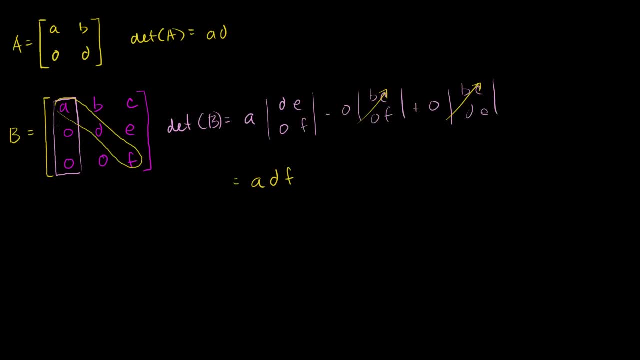 This was the main diagonal right here, And when we took the determinants of the matrix, the determinant just ended up being the product of the entries along the main diagonal, And if you think that that's a general trend that always applies, you are correct. 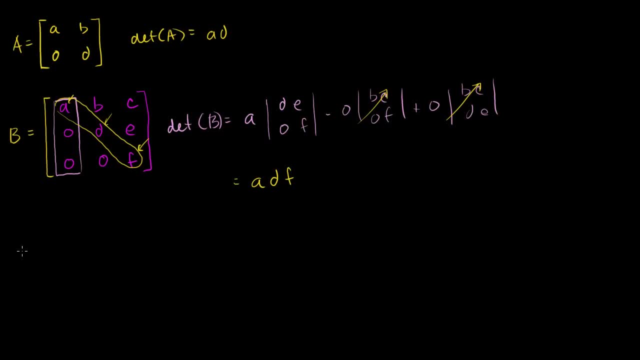 We can do it in the general case. Let's do the general case. So let's say we have some matrix A and it is equal to a 1, 1.. Then you have a 2, 2.. You're going to have a 0, right there. 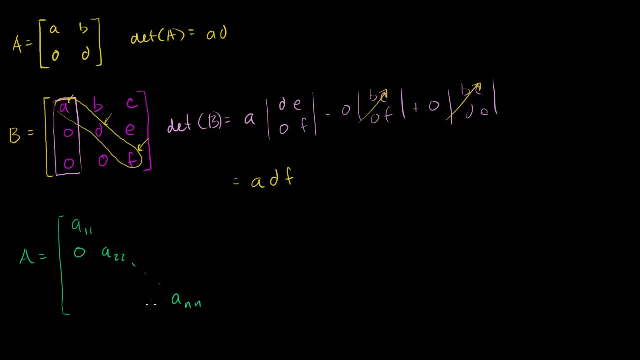 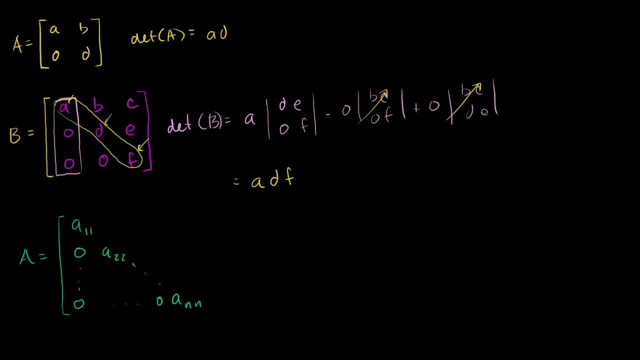 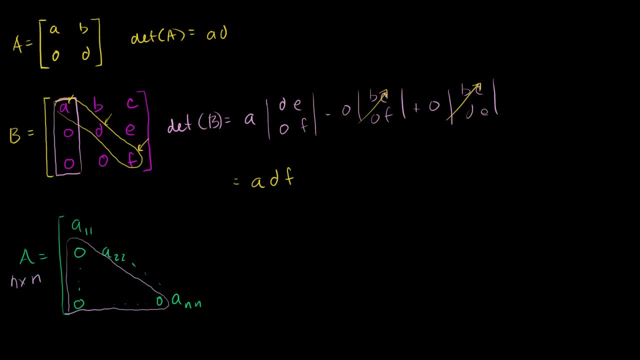 Just like this one, But we're doing it in the general n-by-n case And everything up here is well, it doesn't have to be 0.. This is a12, all the way to a1n. This is a2n. 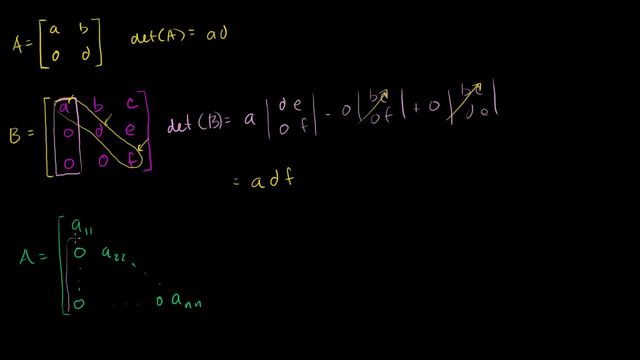 This is all a 0 right here, So everything below the main diagonal is a 0, just like this one, but we're doing it in the general n by n case, And everything up here is well, it doesn't have to be 0. 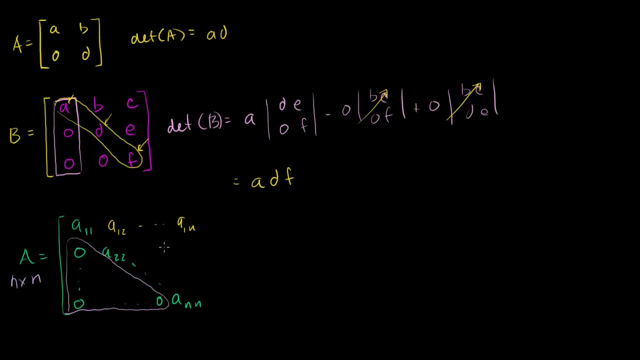 This is a 1, 2,, all the way to a 1, n. This is a 2, n. Keep going down. So everything at the main diagonal or above isn't necessarily equal to 0.. So if you wanted to find the determinant of A, we could do. 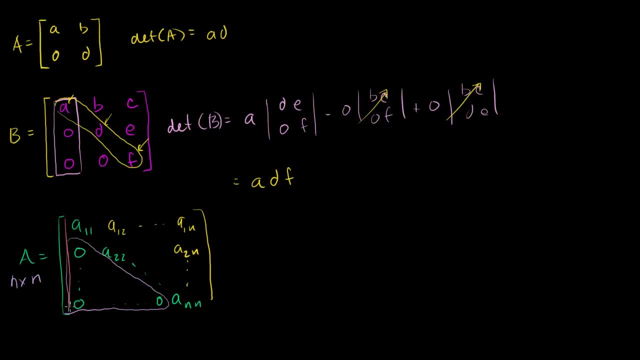 the same thing we did here. We could go down that first row right there. So the determinant of our matrix A is equal to this guy: a 1, 1, times the determinant of its submatrix. So that's going to be a 2,, 2, goes all the way to a 2, n. 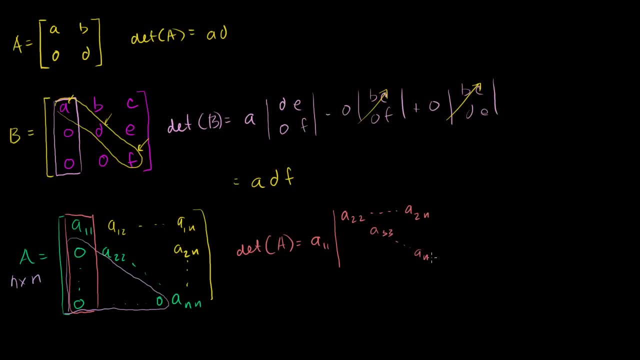 and then a, 3,, 3,, all the way to a, n, n, And then everything down here. these are all 0's, These are all 0's. So once again we have another situation where all of the 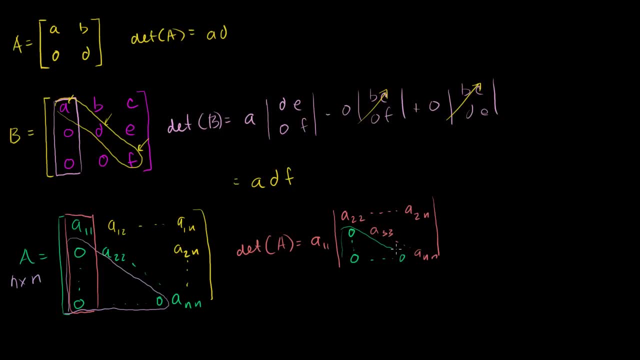 entries below the main diagonal are 0.. So what's the determinant of this guy right here? And you might say, hey, what about the rest of that row? Well, the rest of the row is just a bunch of 0's, just like. 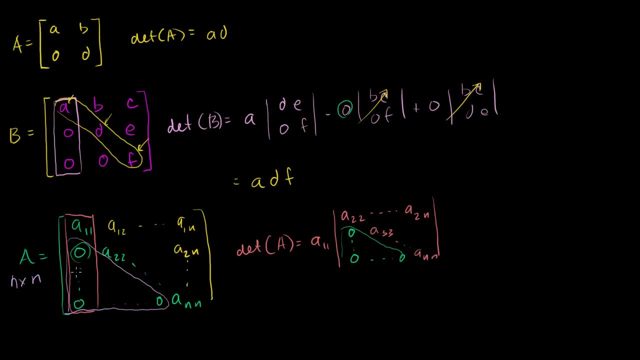 we had here, It's 0 times the determinant of its submatrix, and then that'd be a minus and a plus 0 times the determinant of its submatrix, so on and so forth. So we just have to pay attention to that. 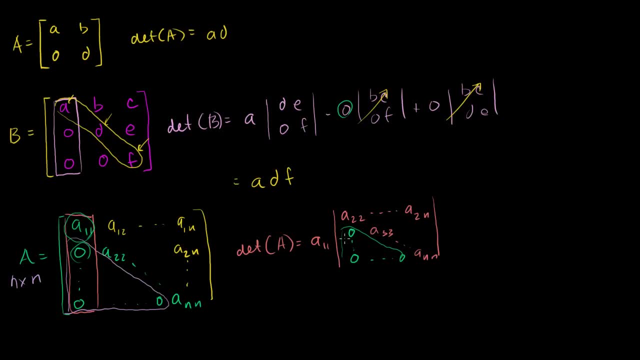 We have to pay attention to this term. right there Now, the same argument we can do here To find this determinant. we can just go down that row. So the determinant of this is just going to be equal to: let's write out, let's not forget our a 1, 1 out there. 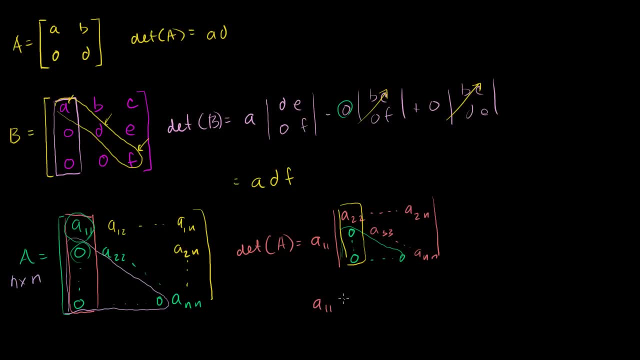 a 1,, 1,, and then the determinant of this is going to be a 2,, 2 times the determinant of its submatrix. Get rid of its row and its column and you're just left with a 3,, 3, all the way down to a n, n. 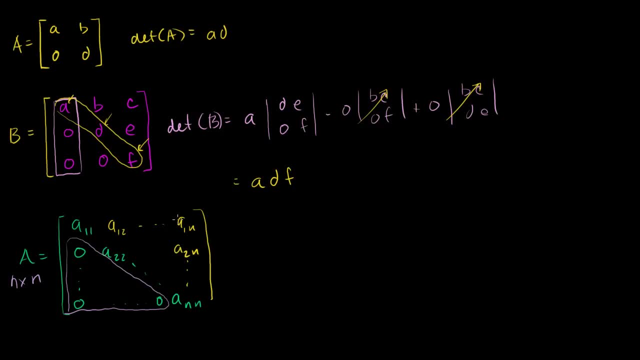 Keep going down. So everything the main diagonal or above isn't necessarily equal to 0.. to 0.. So if you wanted to find the determinant of A, we could do the same thing we did here. We could go down that first row right there. 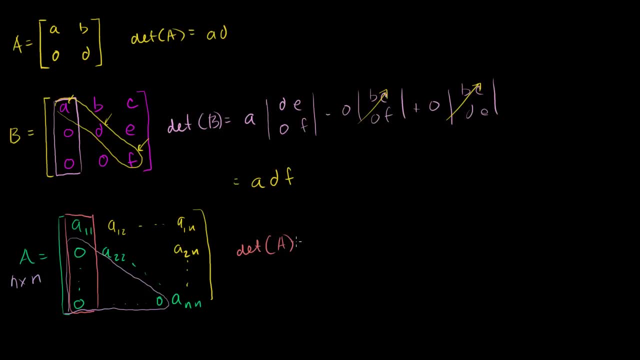 So the determinant of our matrix A is equal to this guy: A11, times the determinant of its submatrix. So that's going to be A22, goes all the way to A2n, and then A33,, all the way to Ann, and then everything down here. 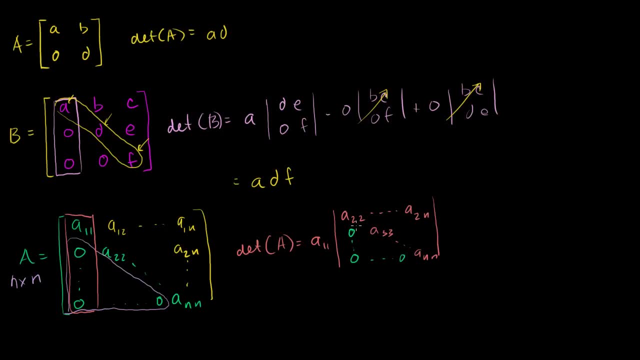 these are all 0's. So once again we have another situation where all of the entries below the main diagonal are 0.. So what's the determinant of this guy right here? And you might say, hey, what about the rest of that row? 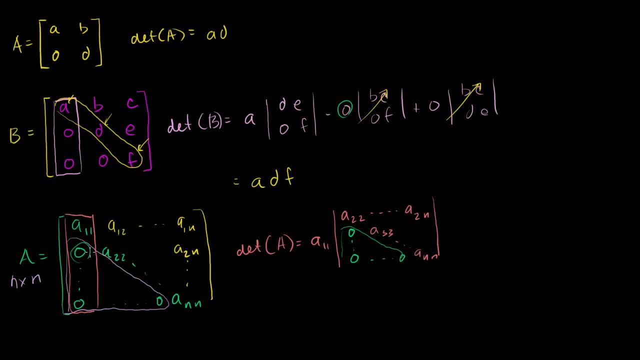 Well, the rest of the row is just a bunch of 0's, just like we had here. It's 0 times the determinant of its submatrix, and then that'd be a minus and a plus, 0 times the determinant of its submatrix, so on and so forth. 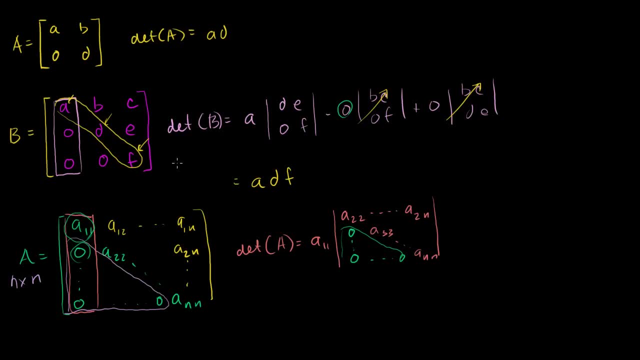 So we just have to pay attention to this term right there Now the same argument we can do here To find this determinant. we can just go down that row. So the determinant of this is just going to be equal to: let's write out, let's not forget our A11 out there. 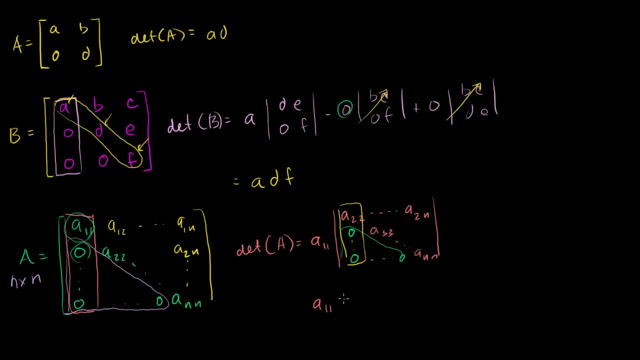 A11, and the determinant of this is going to be A22 times the determinant of its submatrix. Get rid of its row and its column and you're just left with A22.. A33, all the way down to ANN: Everything up here is non-zero. this is A3N. 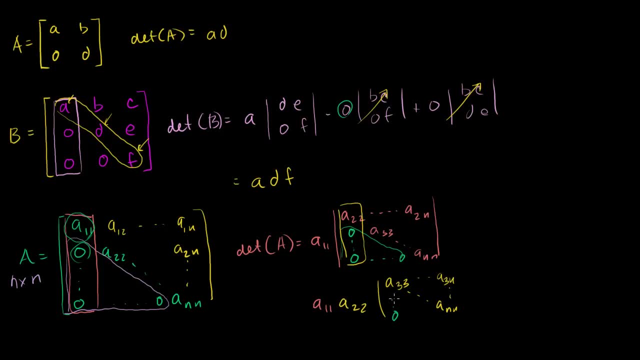 And then everything below the diagonal, once again, is just a bunch of 0's. Everything down here is a bunch of 0's. Another what we call upper triangular matrix. Let me write that down, This whole class where you have 0's below the main. 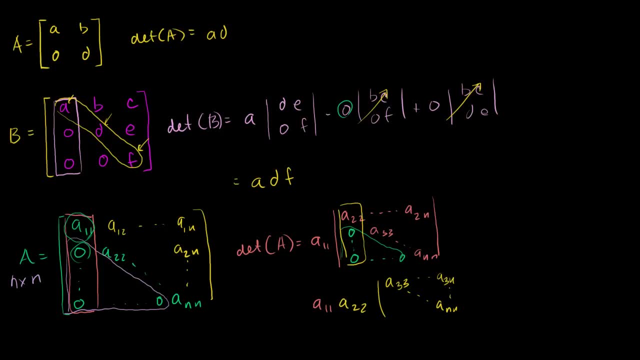 Everything up here is non-zero. This is a, 3,, n, And then everything below the diagonal, once again, is just a bunch of 0's. Everything down here is a bunch of 0's- Another what we call upper triangular matrix. 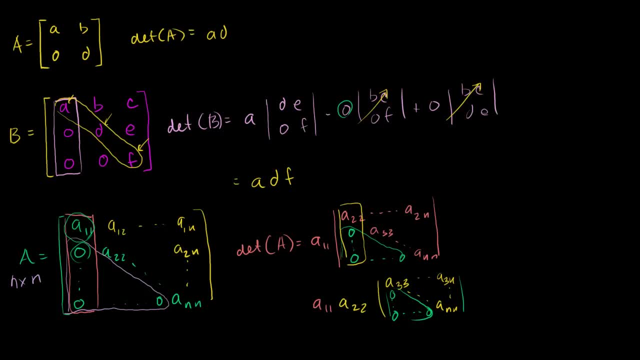 Let me write that down, This whole class where you have 0's below the main diagonal. these are called upper triangular matrices- Triangular matrices, just like that. Now we keep doing the process over and over again. If you just keep following this pattern over again now. 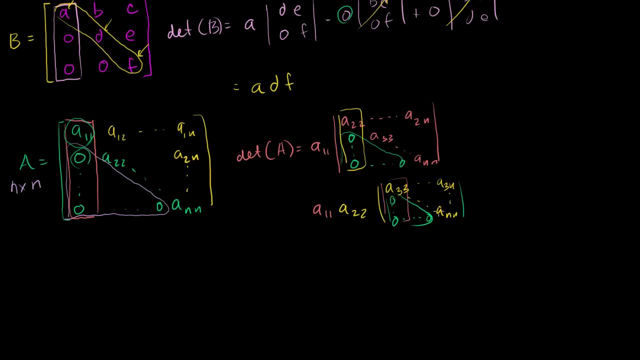 you're going to have. the determinant of this is a 3, 3 times its submatrix, And every time the submatrix is getting smaller and smaller, you will eventually get to a 1, 1 times a 2, 2. 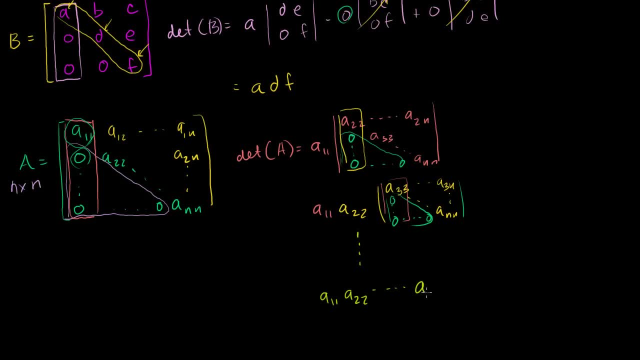 times all the way to a n-minus 2, n-minus 2, times a: 2 by 2 matrix over here: Times a 2 by 2 matrix here That's just going to be a n-minus 1, n-minus 1, a n. 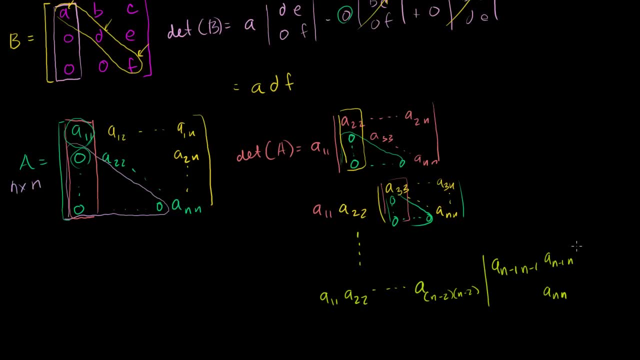 sub n. This is going to be a sub n-minus 1, n, And then you're going to have a 0 right here. So it's just the bottom right-hand corner of our original matrix is what you're going to be left with. 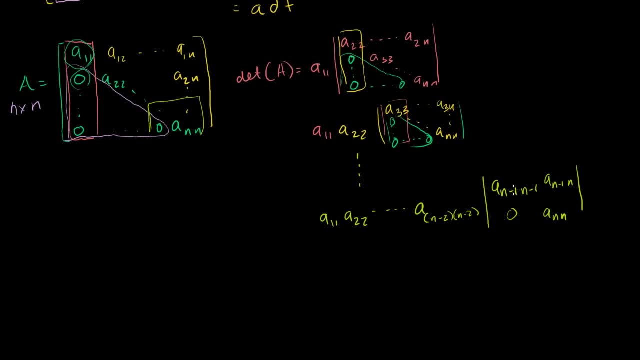 And what is the determinant of this? Well, it's just the product of these two things: This guy times this guy minus this guy times that guy, But that's just 0.. So the determinant of a ends up becoming a 1,. 1 times a 2,. 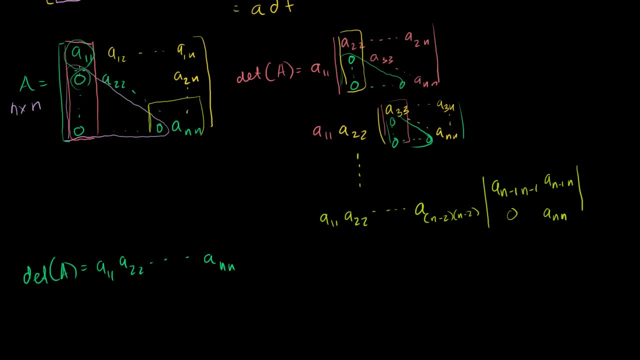 2, all the way to a, n, n, Or the product of all of the entries of the domain diagonal, which is a super important takeaway Because it really simplifies finding the determinants of what would otherwise be really hard matrices to find the 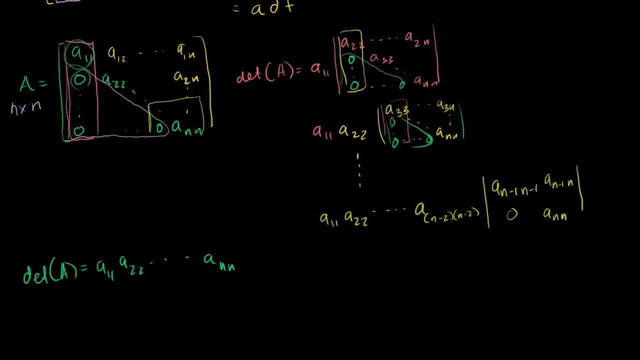 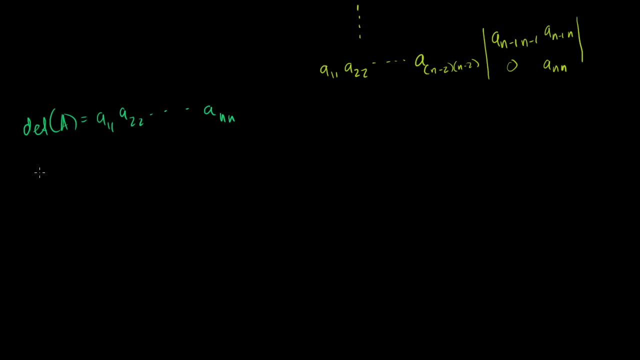 determinants of. You could imagine if this was a 100 by 100 matrix, You could just multiply the diagonal. So just to make sure that things are clear, let me do an example. Let's say we find the determinant of 7,, 3,, 4,, 2.. 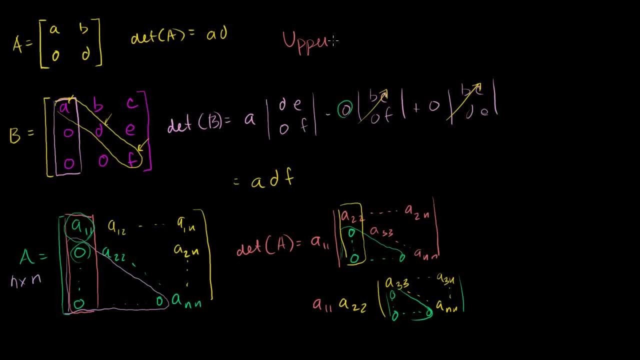 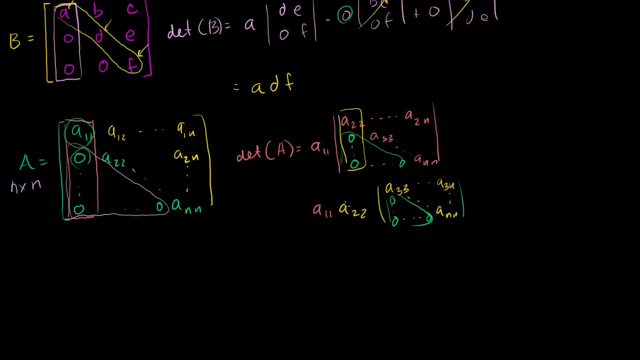 diagonal. these are called upper triangular matrices- Matrices just like that. Now we keep doing the process over and over again. If you just keep following this pattern over again now you're going to have: the determinant of this is A33 times its. 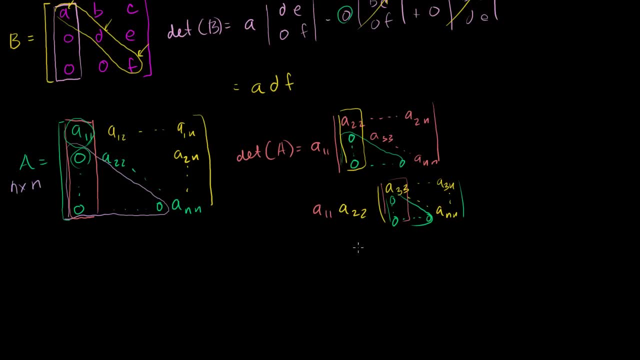 submatrix, and every time the submatrix is getting smaller and smaller. you will eventually get to A11 times A22, times, all the way to AN minus 2.. AN minus 2. Times a 2 by 2 matrix over here. 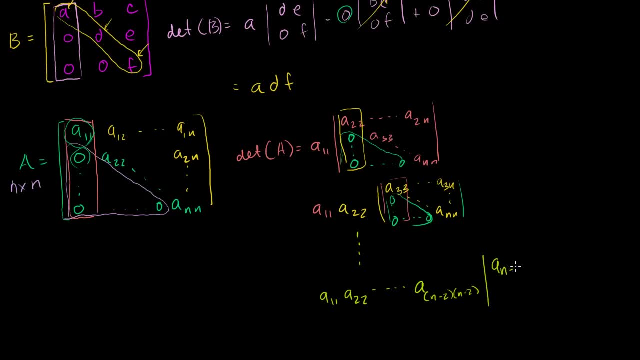 Times a 2 by 2 matrix. here There's just going to be AN minus 1, AN sub N. This is going to be A sub N minus 1N, And then you're going to have a 0 right here. 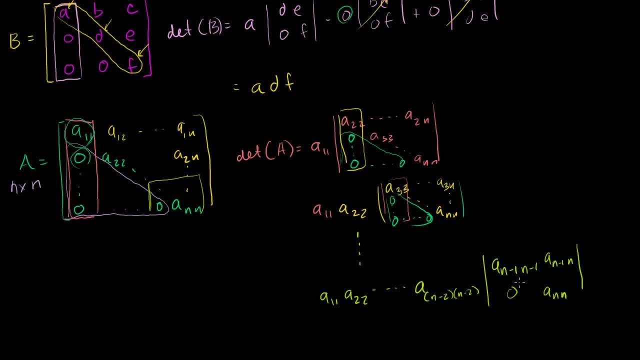 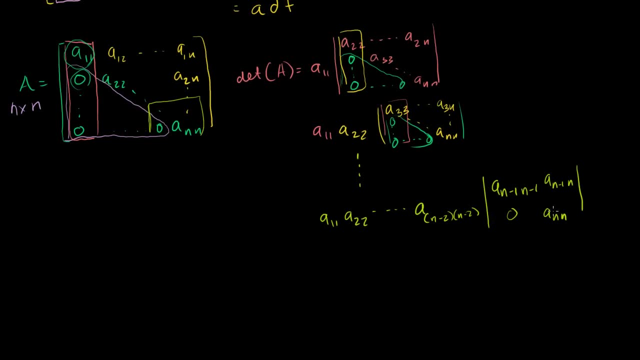 So it's just the bottom right-hand corner of our original matrix is what you're going to be left with, And what is the determinant of this. Well, it's just the product of these two things. It's just this guy times this guy minus. this guy times that. 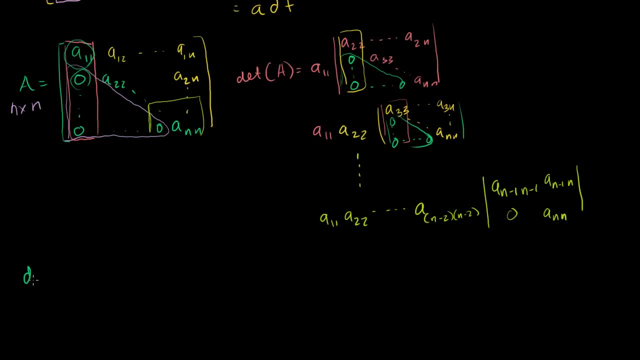 guy, but that's just 0. So the determinant of A ends up becoming A11 times A22, all the way to ANN, or the product of all of the entries of the domain diagonal, which is a super important takeaway because it really simplifies finding the determinants of. 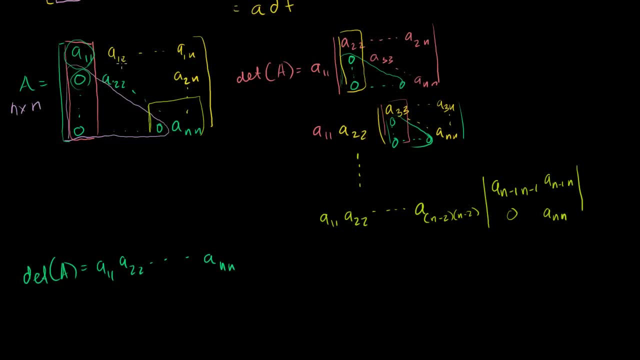 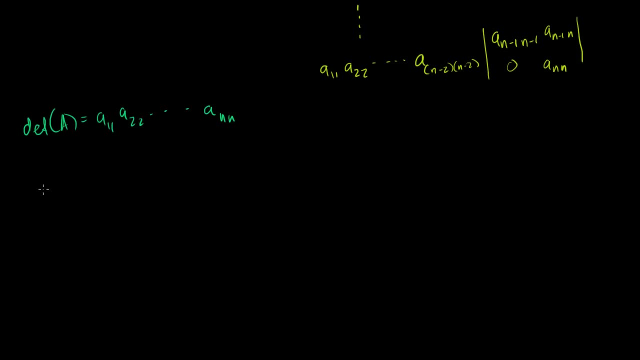 what would otherwise be really hard matrices to find the determinants of. You could imagine if this was a 100 by 100 matrix. Now we can just multiply the diagonal. So just to make sure That things are clear, let me do an example. 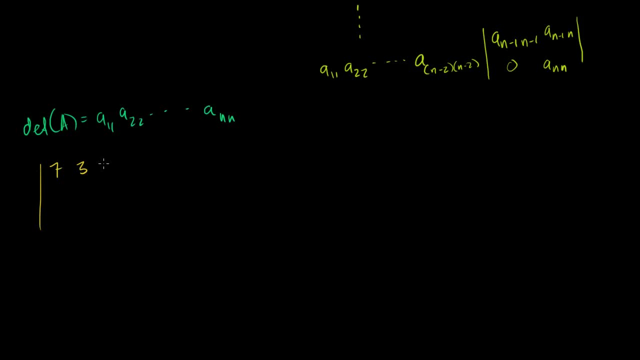 Let's say we find the determinant of 7,, 3,, 4,, 2.. Yes, so we have 0's here. Let's say it's a minus 2,, 1, and a 3. We have a 0 here. 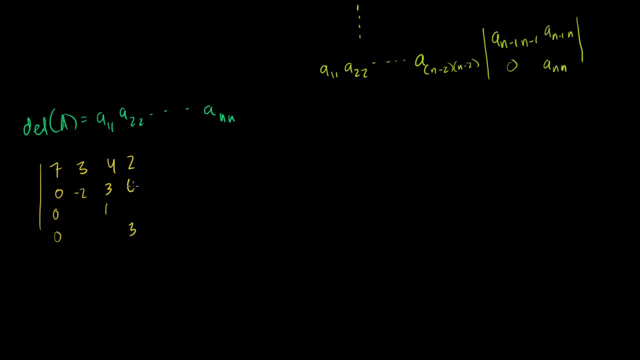 Sorry, we don't want 0's there. We don't need to have 0's there. 6, 7.. We actually could have 0's there, but we don't need to have 0's there. You have a 0 there and you have 0's there. 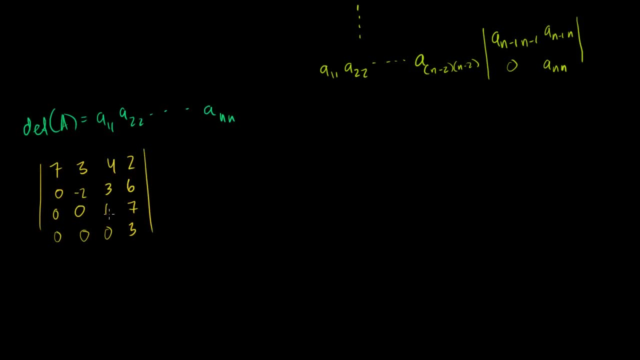 Just like that. So it's upper triangular matrix. If you want to evaluate it, you can do that. If you want to evaluate this determinant, you just multiply these entries right here. So the determinant is equal to 7 times minus 2 times 1 times.